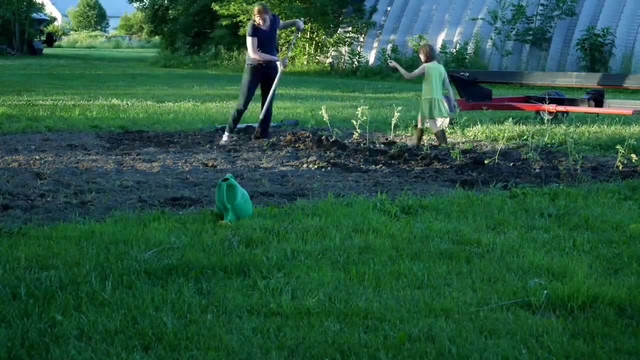 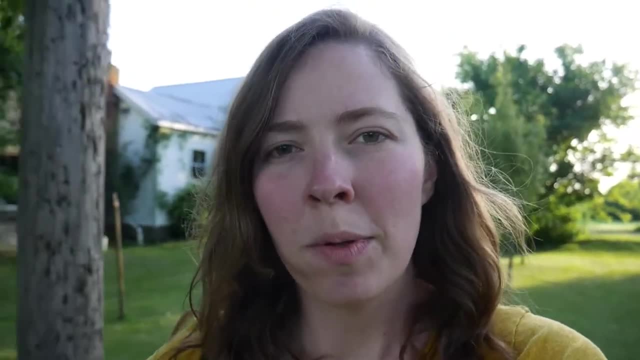 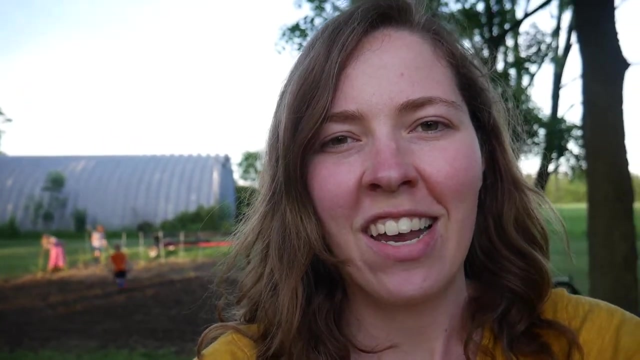 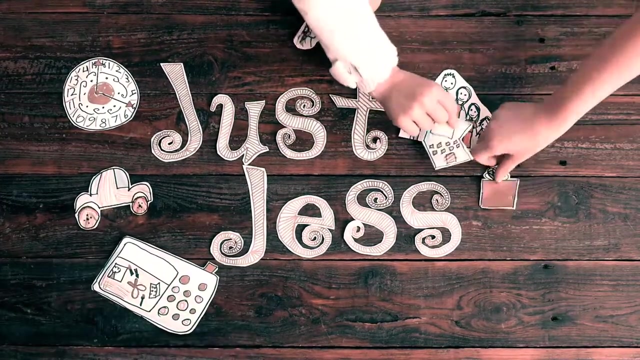 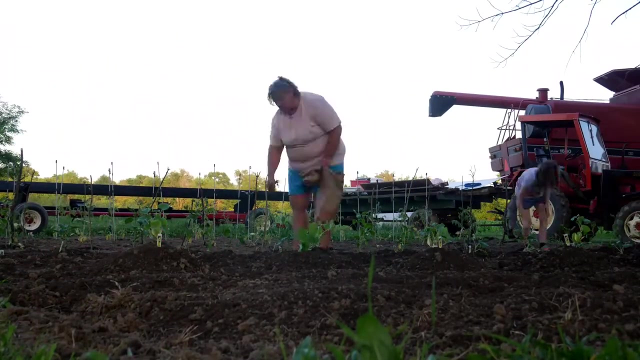 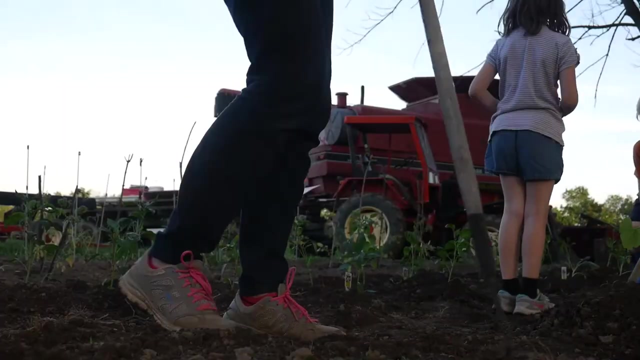 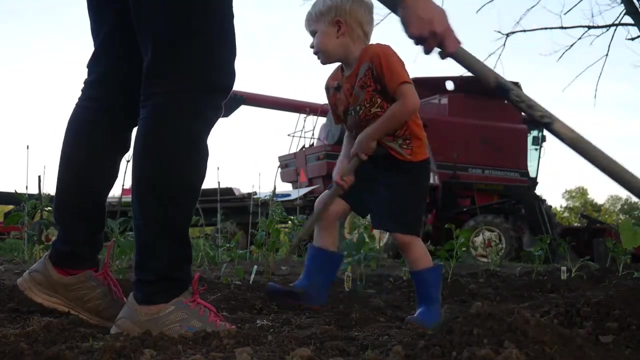 We are going out to work on our garden today. We planted the tomatoes the other day and now we have the rest of the vegetables to plant. So you see my kids out there getting a head start already, So let's begin the process. Well, that's good, It will fill out the rest of this row. Yeah, There's going to be kind of an empty spot right here if we didn't have that, so 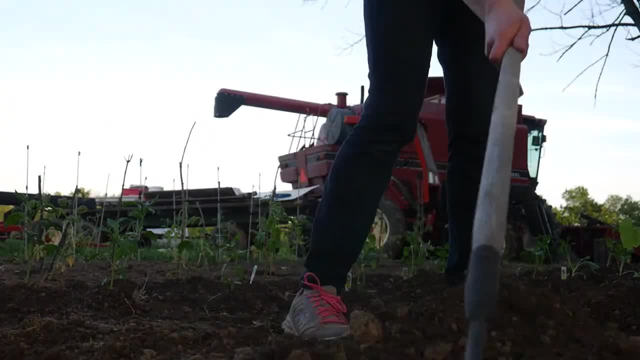 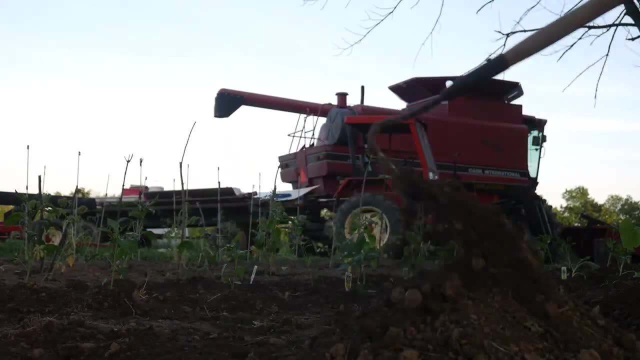 We need the seed, or else it wouldn't be there. Alright, who has the plant? You have it. Are you going to plant it this time, Annabelle? Yeah, Yeah, Yeah. Can I use this for little fairy houses? I suppose you could. 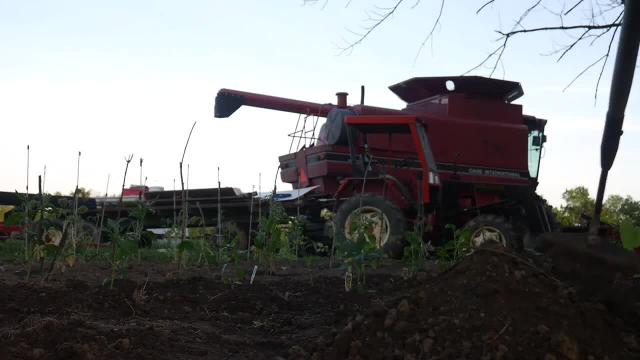 It's not like they could hurt anything. No, no, no, Alright. Who's going to dig the hole? I'm going to dig the hole. You're going to dig the hole. Careful, Yep, Let me. Oh, you're going to do it, Okay. 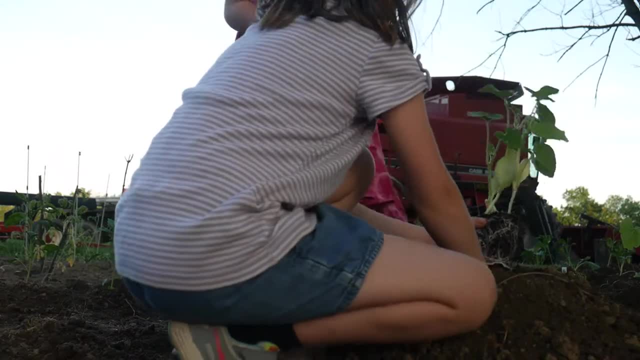 Alright, And you get to drop it in Annabelle. There you go, Thank you. Can you put this in the wagon for me? Here's your tag. Here's your tag, Abby. I'm going to pat it down. You want to put the tag with it? 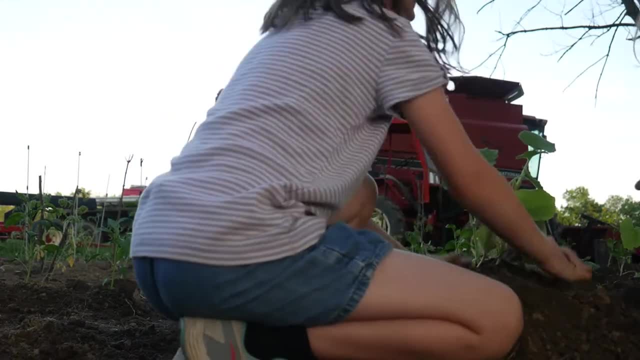 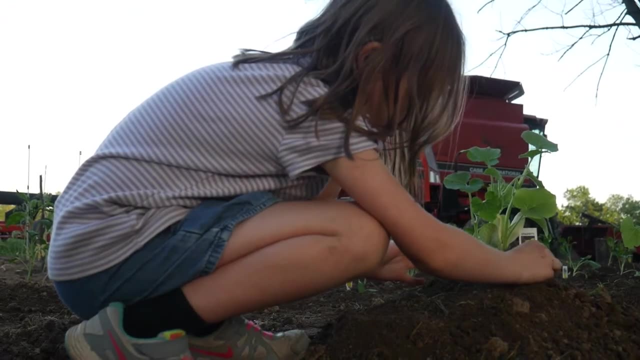 Oh sure, That way we know where it's going to go. I'm going to put it in the wagon. Here's your tag. Here's your tag. Now we only have seeds. Go ahead, Abby. Can you pick that up for Momma? 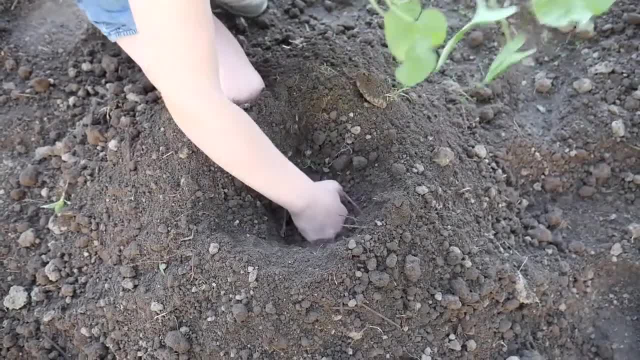 I don't feel like I do with my help. Well, you are actually. You got clean. That's all this one's for. I don't want to be hoarding the seeds. You got to dig a nice deep hole, huh. 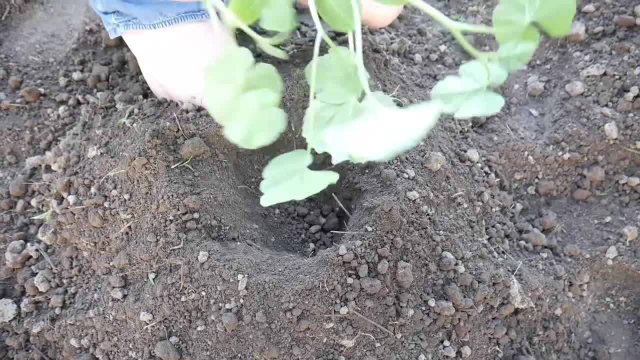 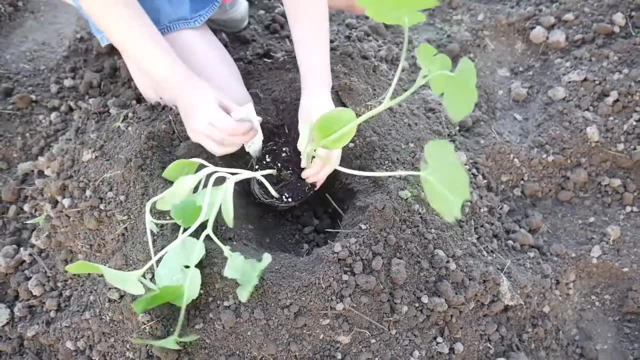 So the roots will be good- Uh huh, And down there, Yeah. And then if we water them too much, the dirt will extra soak it up and then the roots don't get too much Mm. hmm, Ivan, don't swing around that hoe. 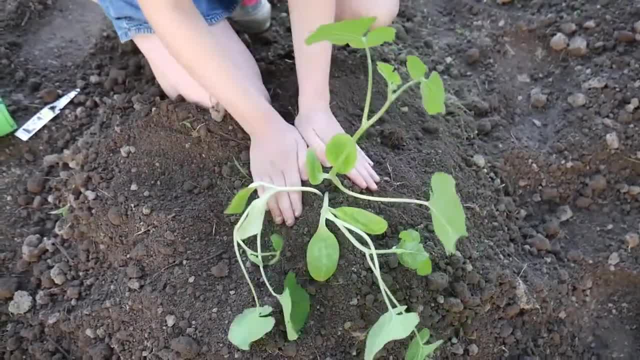 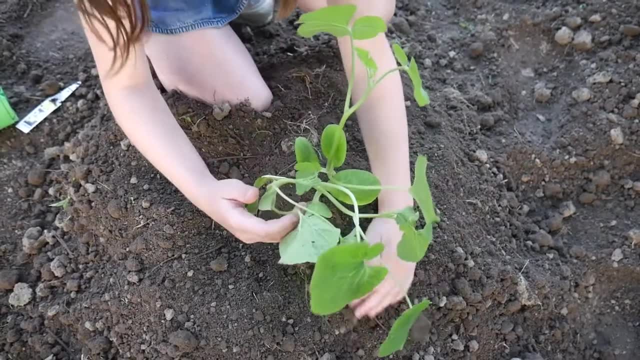 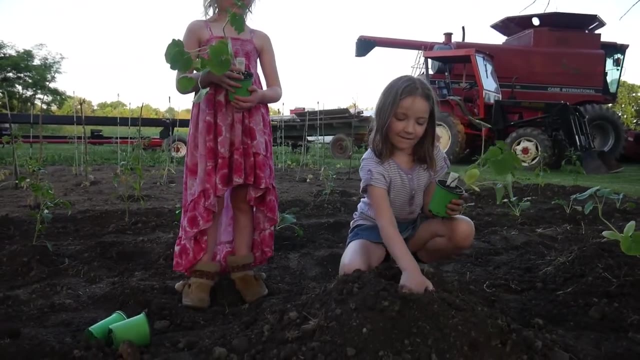 See, Make sure it gets lots of dirt around it to support it. Nicely done. You could do a little more around it. maybe There you go. Careful Arva, What? What kind of plant is that, Abigail? 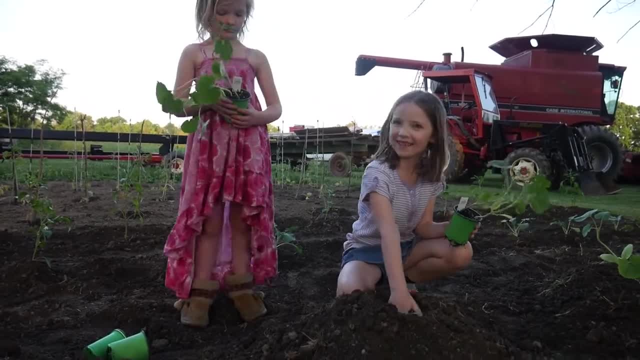 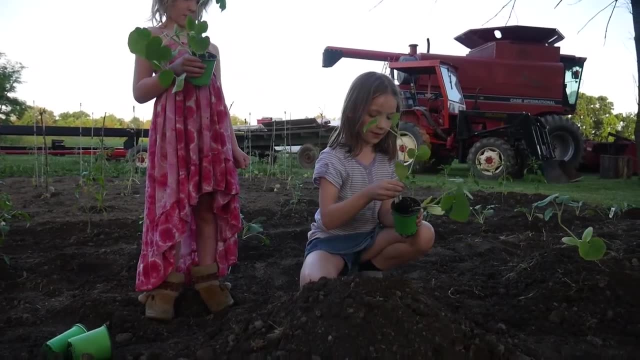 It says You need to put that down. Squash- Is that good? Spaghetti squash? Yes, Ooh, spaghetti squash Sounds yummy, Mm-hmm. Let's see if I can get this plant out. So there are noodles inside of it that actually cross. 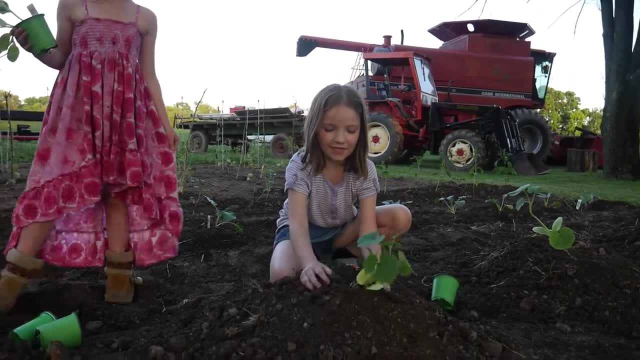 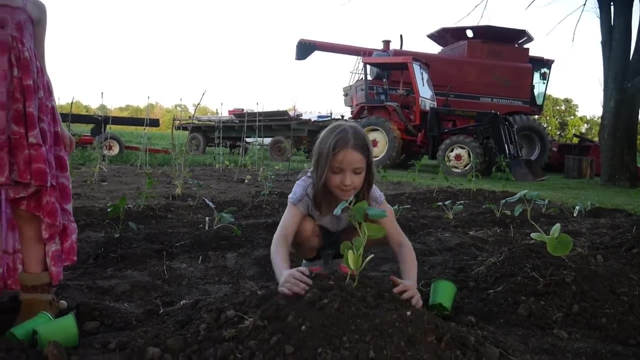 Yeah, Is that what it is? I don't think whatever she said is correct, Actually, yeah, you can eat it like spaghetti. You cook it up and you shred it and then you can put pasta sauce on top of it. Yeah, we had that before. 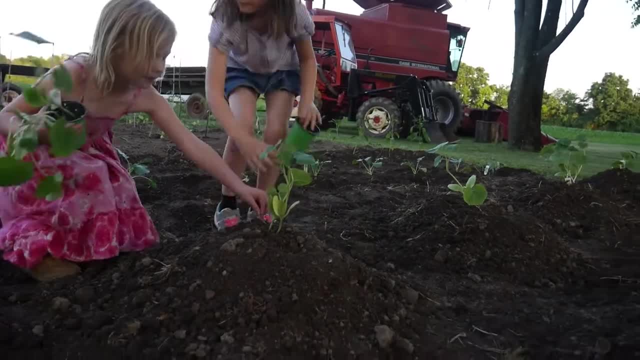 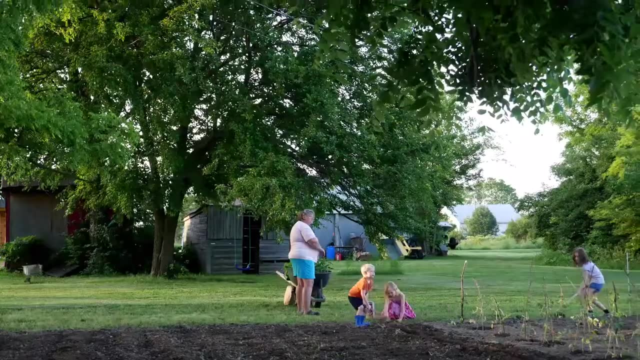 Remember Mm-hmm, I'll be the top of mine. Okay here, Okay Here, This is the top. I'm going to take it off. Okay, I'm going to take it off, You don't have to. 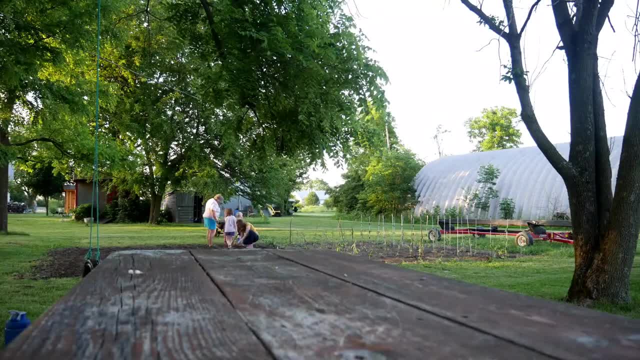 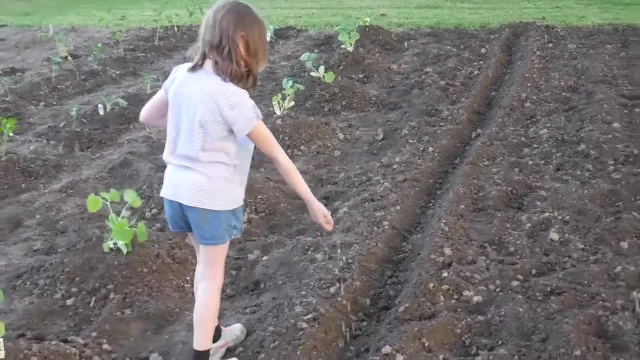 I'm going to take this off, Okay, Okay, I'm going to be the top, Okay, All right. All right, Good job. You guys are doing a great job. Thank you, You're welcome. All right, Thank you guys. 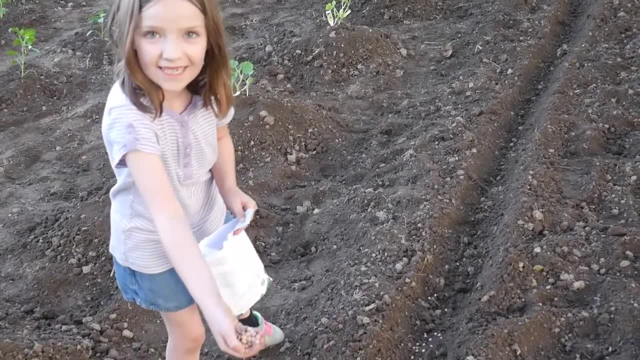 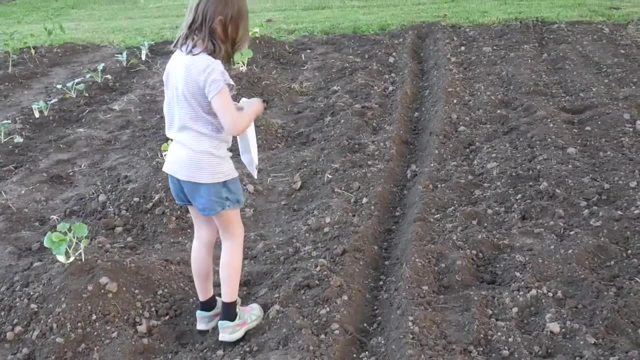 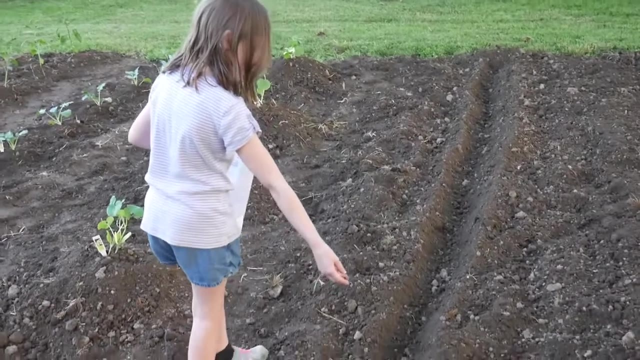 Have a great day. Bye-bye, Bye-bye, Bye, Bye-bye, Bye-bye, Bye-bye, Bye-bye, Bye-bye, Bye-bye. Well, I would think pink, pinkish, red pea seeds- uh, that that sounds weird really. 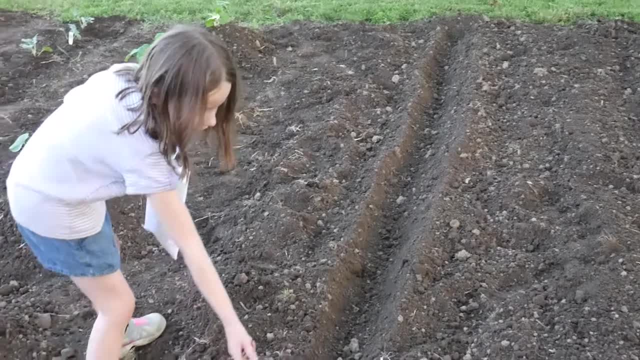 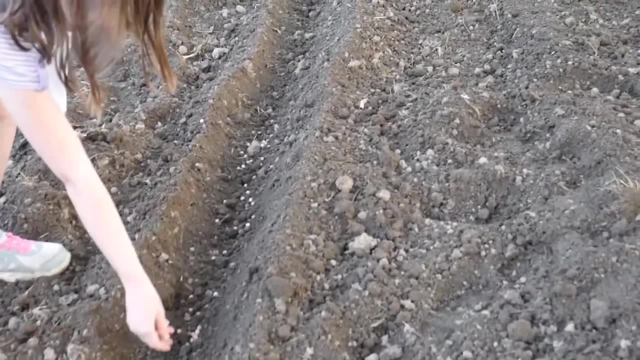 weird, Sounds a little weird. Yeah, I would think it's weird. Oh yeah, I missed a little spot. Try to do it evenly. Okay, There you go. Wow, It's just kind of like feeding the birds, Mm-hmm. 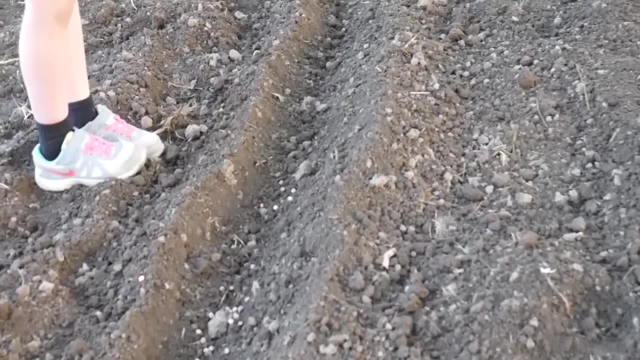 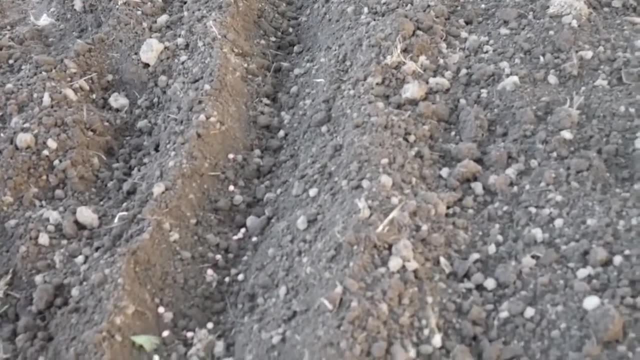 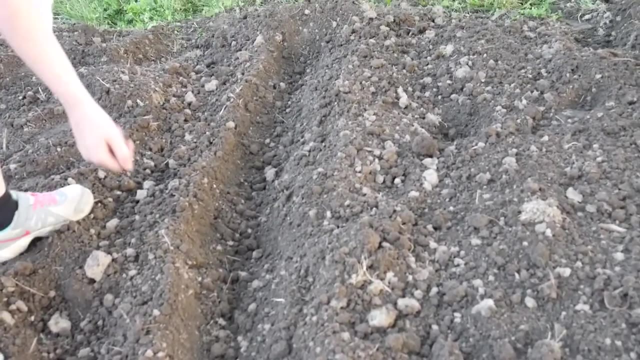 Peas are kind of viney. They like growing on each other, so they'll turn into a big Patch. It'll look like a big bush. Yeah, it will. Of a bunch of beans, A bunch of peas, Yeah. 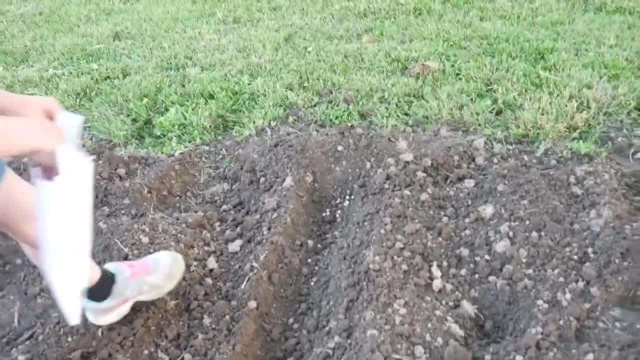 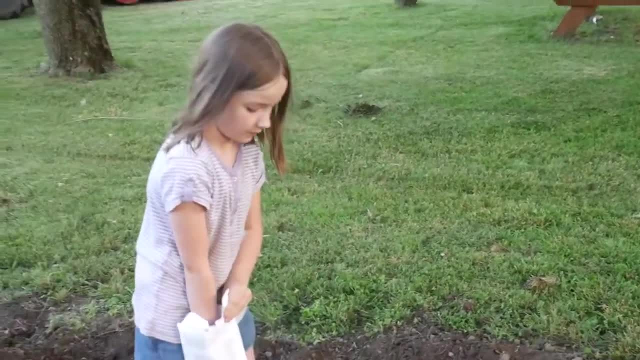 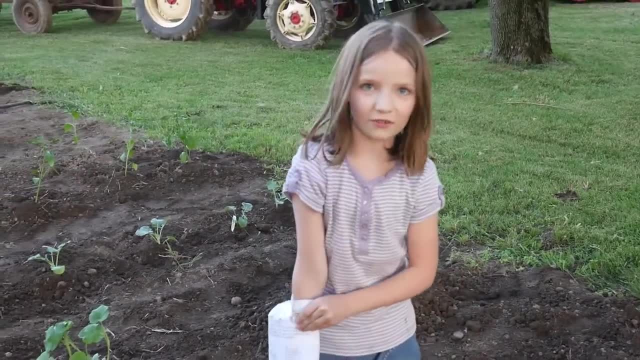 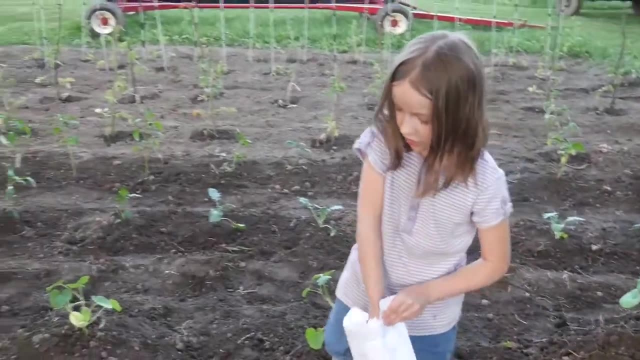 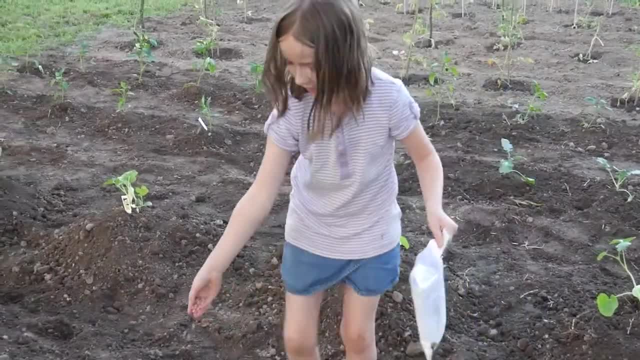 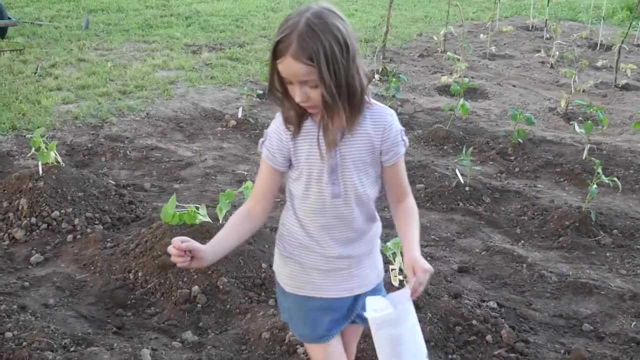 Mm-hmm, Look at all these pea plants we're going to have. I do not eat peas- Not one. You might like them when they're fresh out of our own garden. I may, actually I may- eat them because I actually I rather have food that's actually running on my own. 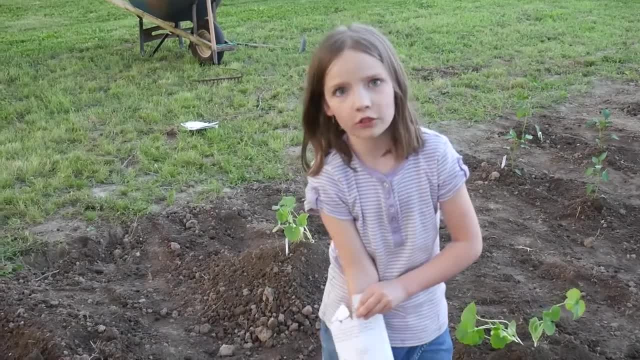 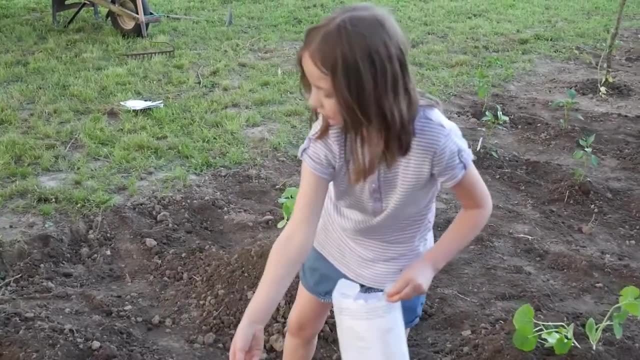 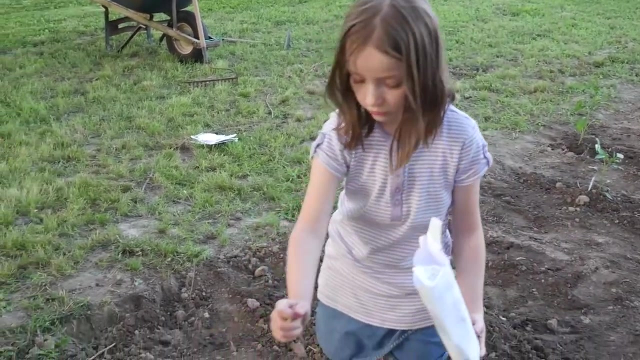 I like my peas. I love peas, actually from our own garden and from our own home and made especially by us. Tastes a lot better. Tastes more homemade? Oh yeah, I think so. huh, Home grown Yeah, Home grown yeah. 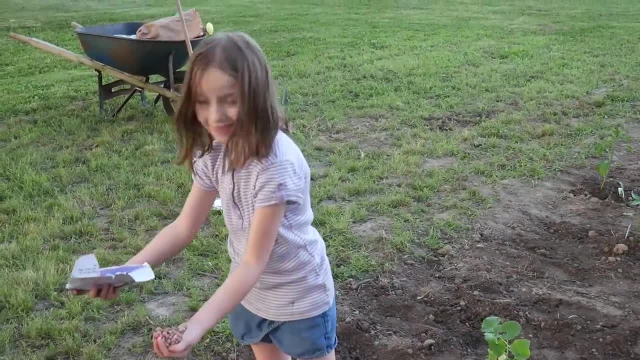 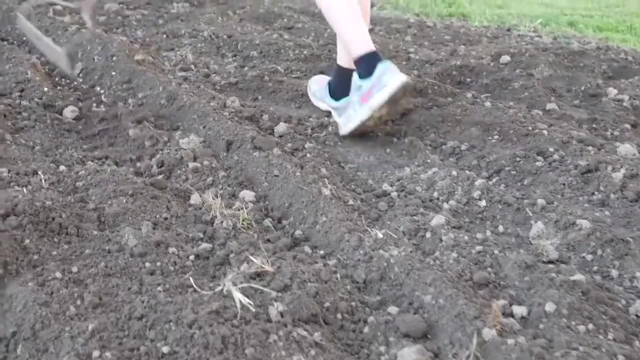 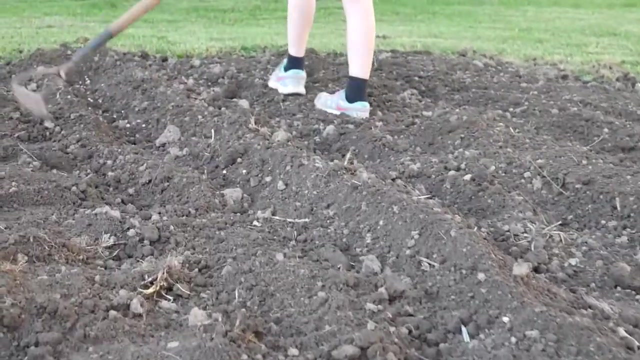 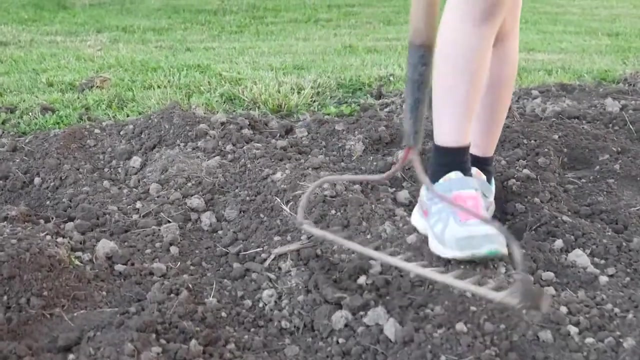 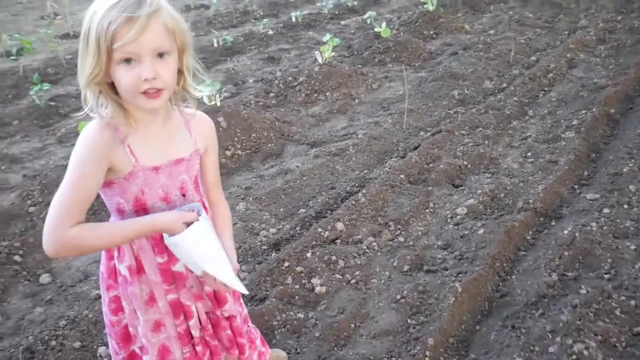 There's a couple more left. Oh, that was quite a few, But it needs lots of water, Needs lots of water. huh, For your one little onion, Annabelle. Yeah, Here we go. What are you planting, Annabelle? Peas, Peas. Yeah, we decided to do a second row of peas, huh. 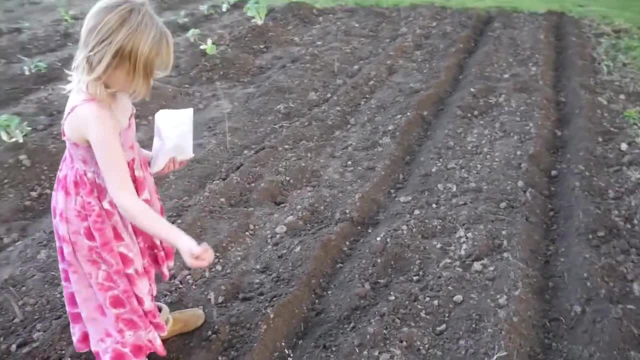 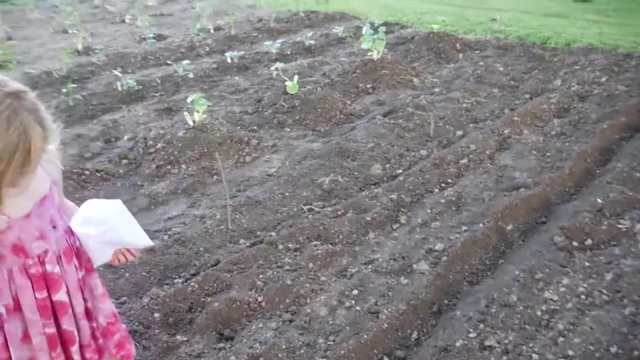 They are pink. They are pink. Some of them are a little green. Yeah, You want to plant them like this type? I'll let you know here in a second. Yeah, they're pink because that keeps the bugs from eating them. 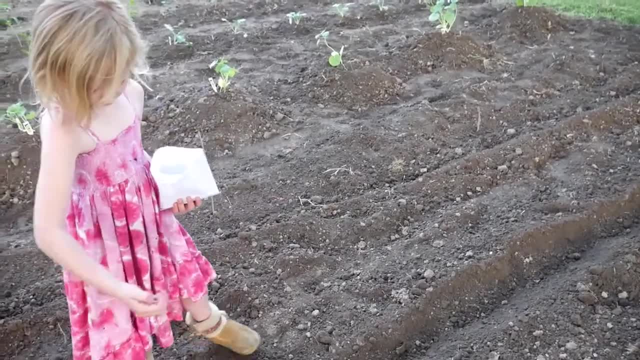 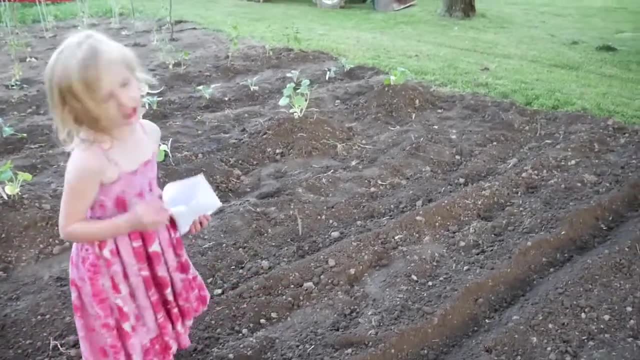 You put powder on them so that bugs and animals don't want to eat them Because they smell bad to the animals. but they smell good to us and we can eat those type of chemicals. Well, no, we don't eat them. They grow into plants and then it washes off over time. 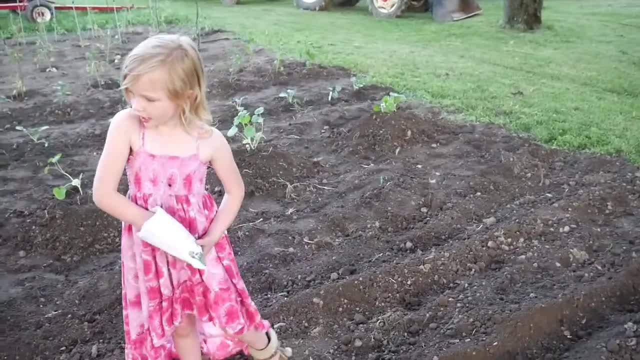 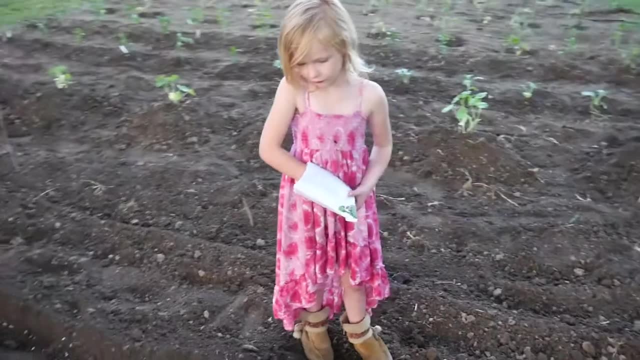 Yeah, Because the dirt damp make it kind of get very moist and wash away the poisonous. Yeah, Oh, look at this, While you're putting them down, Abigail's raking them over. Well, that's speedy. It's a good, speedy way of doing it.